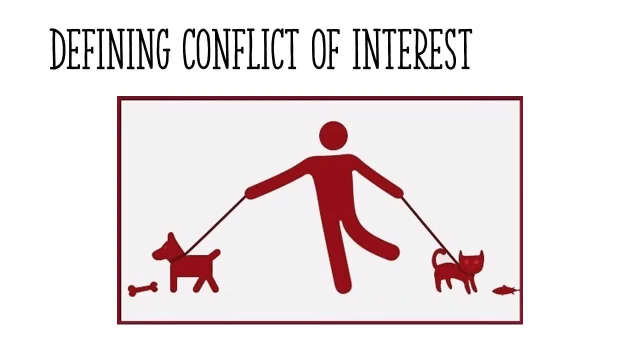 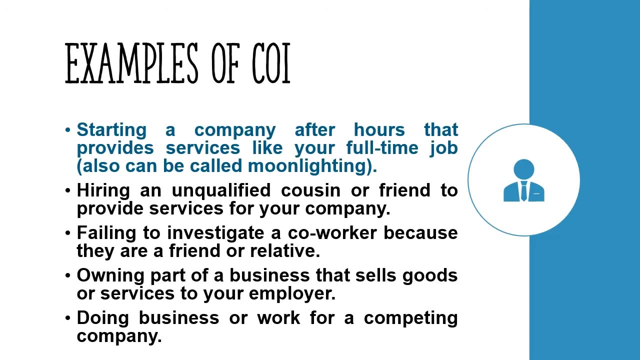 If you feel you are being put in a conflict of interest-inducing situation, state your conflict and avoid the situation altogether. Let us look at some examples of conflict of interest. Let's say you have a startup and a full-time job, both in the same field. 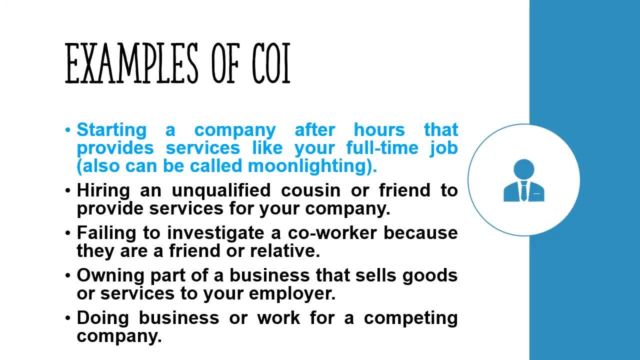 This means that your startup may have access. You may have access to your work's data and deals through you, and this may lead you to do some bad decisions. Another case is when you are in charge of hiring at a company and a friend or family member applies for a vacancy. 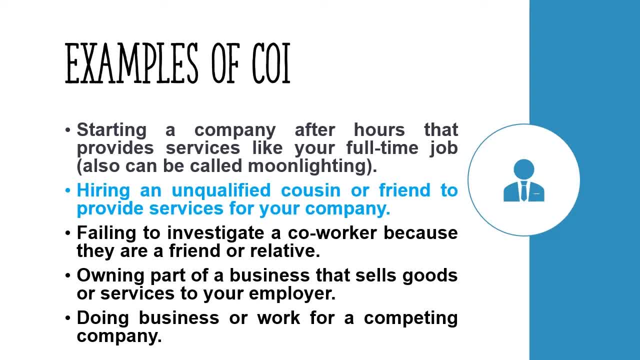 If they are unqualified and they don't get hired. this may lead to social troubles and may have you inclined to help them out. It is better to avoid the situation and let someone else interview that individual. The same goes when you have to double-check the work of a friend or a relative. 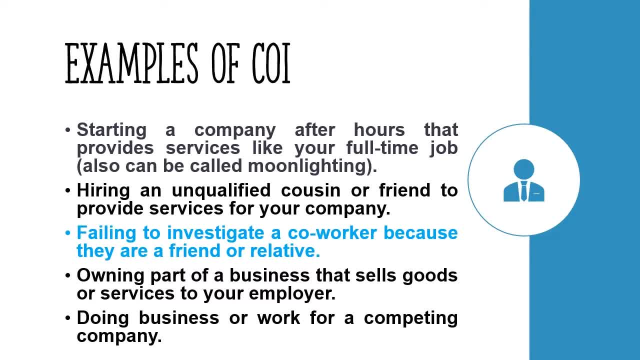 You might be tempted to cut them some slack as well, and this is also unacceptable. Another example is owning a company that provides essential goods or services to your employer where you work full-time. It isn't hard to argue here that a person might be tempted to improve their profits on both ends. 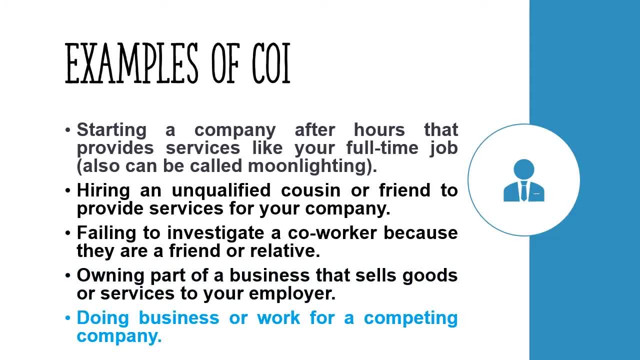 The final example here is receiving money to do work for a company that is a competitor to your full-time employer. This not only poses a question of whom to give an edge to, but also might cost you your job. These were a few of many examples on conflict of interest. 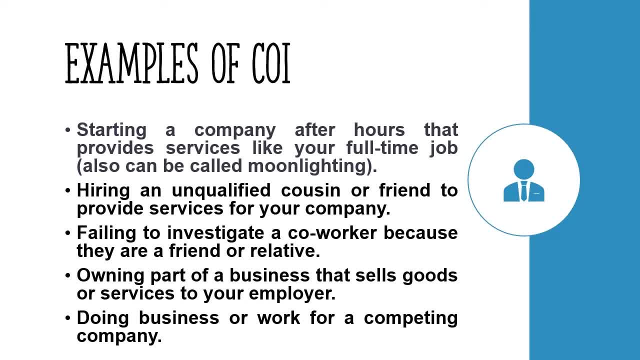 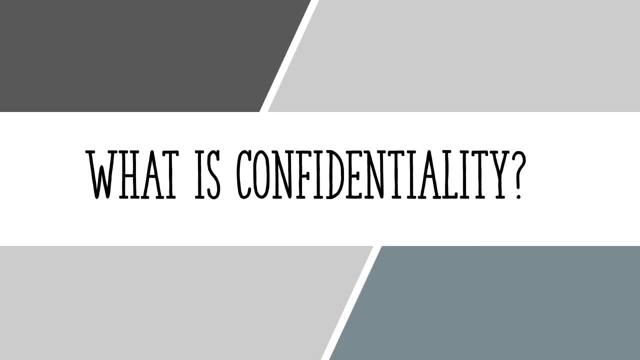 What examples can you think of? Write them down in the comments below. From conflict of interest we move on to confidentiality, a topic that you might have heard of, especially in movies. What is confidentiality to you and what are your experiences with it? 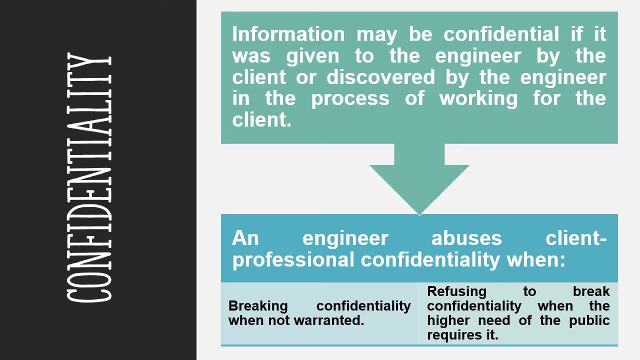 The information that you gain through your work is generally confidential. That is why it is highly expected of you, as a professional, to keep it secret, and to yourself. Giving out this information with no cause is considered an abuse of confidentiality and may leave a smear on your career.